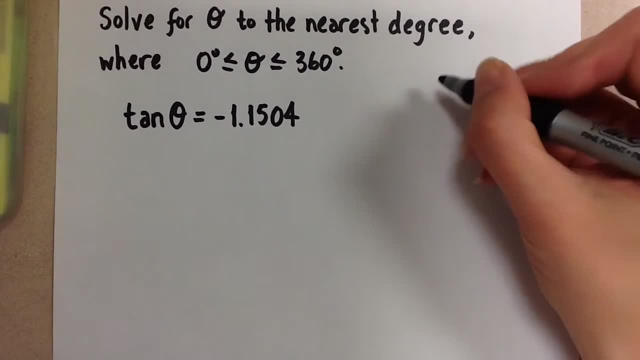 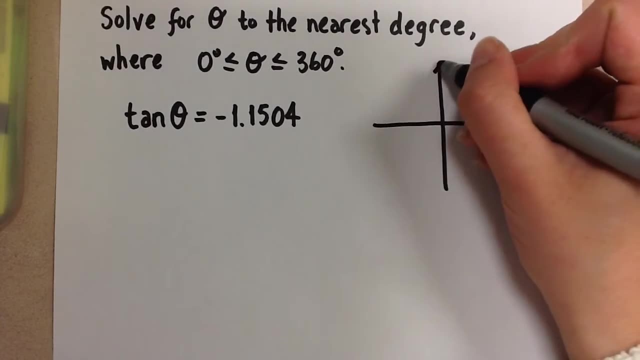 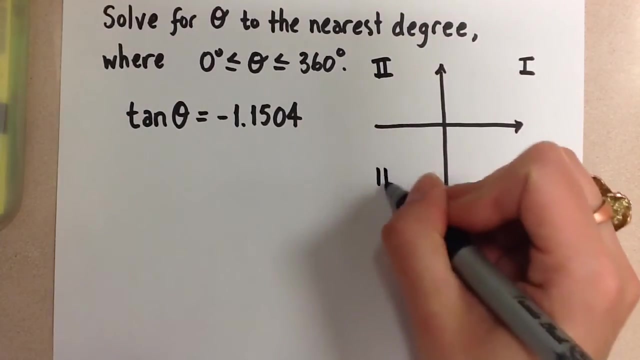 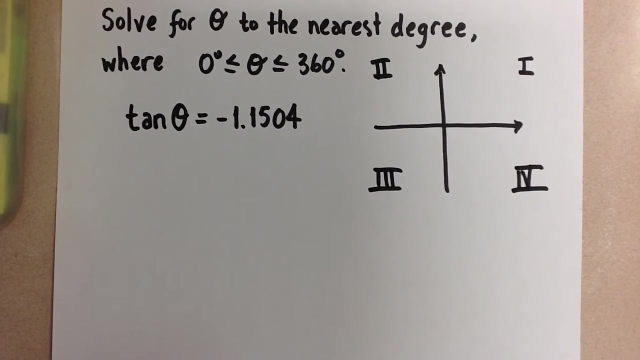 So to do this, we have to remember our cast rule. So let's refer back to that. If we have the Cartesian plane here like this, our quadrants are 1,, 2,, 3, and 4. And our cast rule says that the trig ratios are: 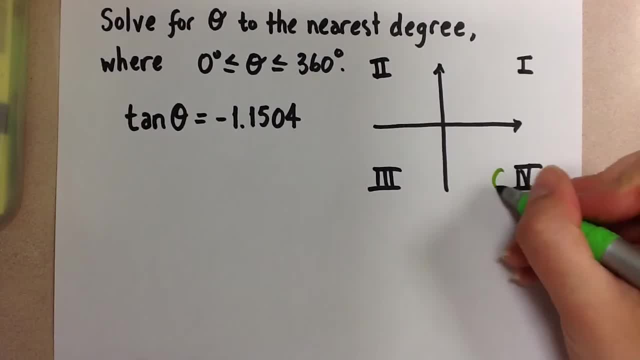 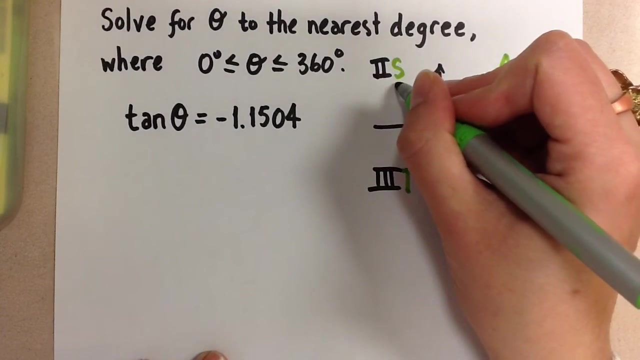 positive, positive in these quadrants. So there's our cast acronym. This means that in the fourth quadrant, the cosine ratio will be positive. In the first quadrant, all of the ratios will be positive. In the fourth quadrant, the sine ratio will be positive. 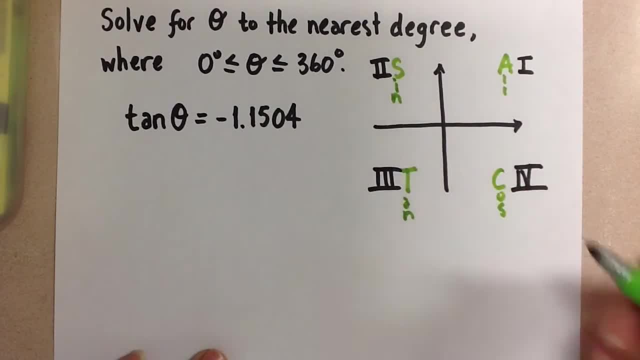 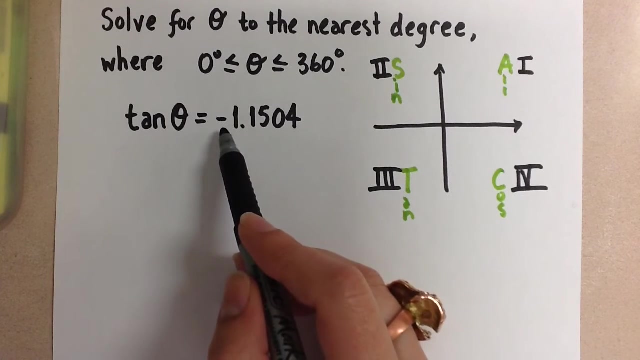 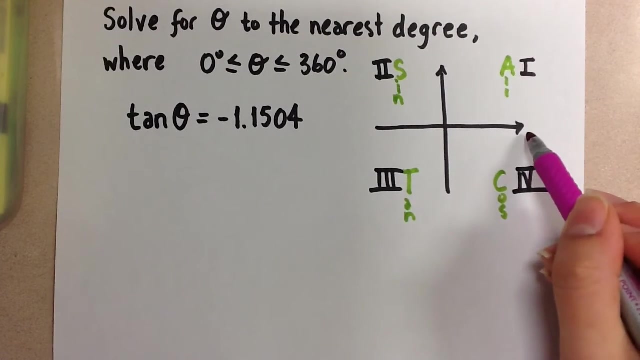 And in the third quadrant the tangent ratio will be positive. So that's what our cast rule says. So when we're solving for this particular angle in this equation here, we see that the tangent of the angle is negative. So this means we're going to be working in the fourth quadrant and in the second quadrant. 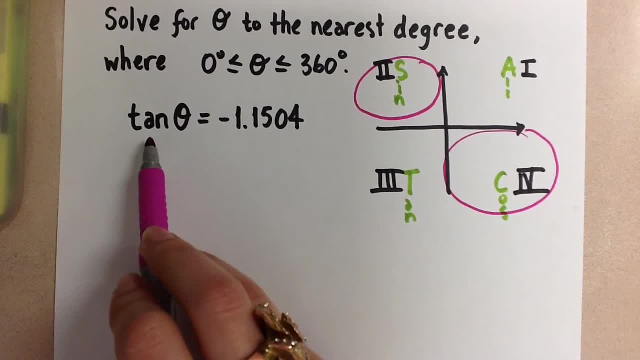 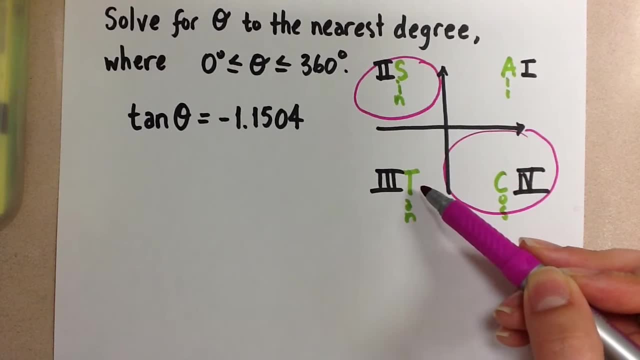 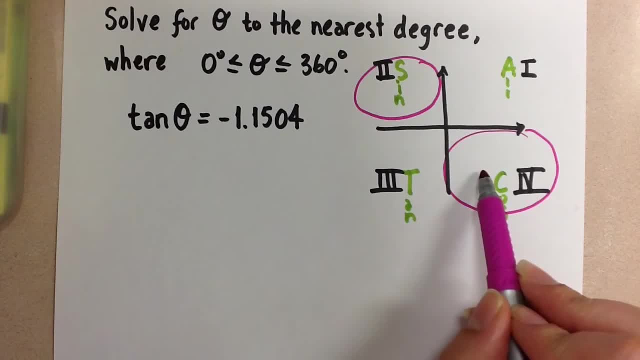 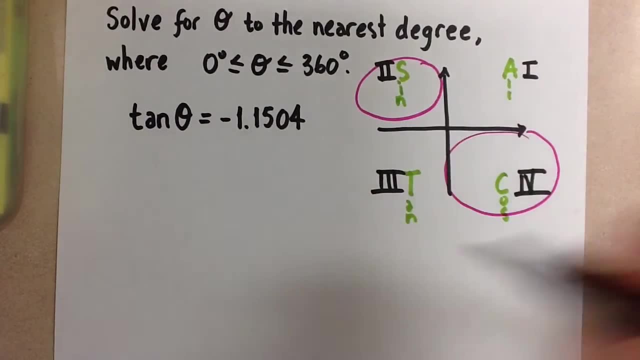 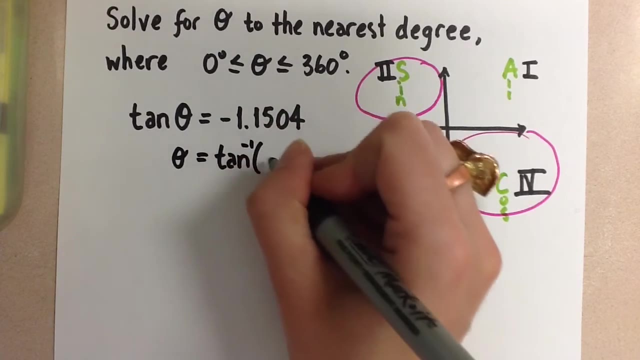 So we know the two angles we're going to find are in the fourth and in the second quadrant here. So the first thing we want to do is solve for angle theta here using the inverse of tangent. So we do this on our calculator to solve. 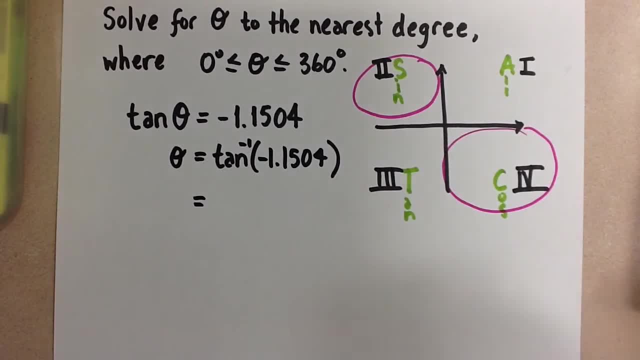 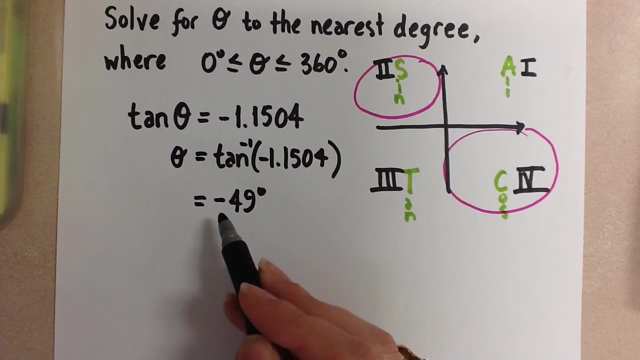 For theta, And when we do that, we're going to get negative 49 degrees. Now, this is a negative angle, but we can still work with this. We don't when we calculate our trig ratios on our calculator. we don't always get positive angles. 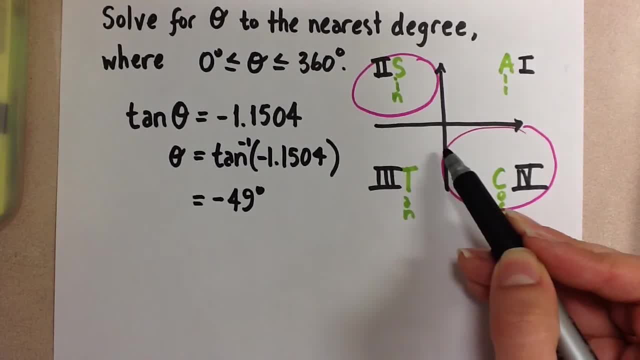 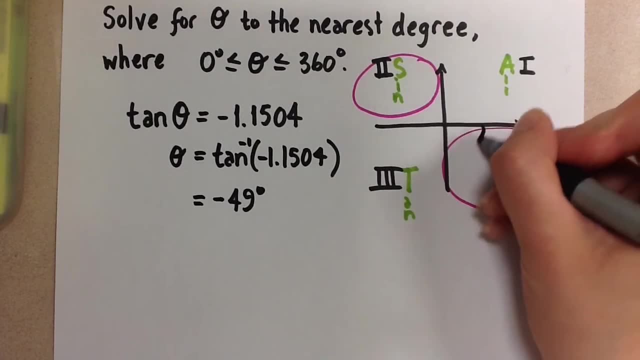 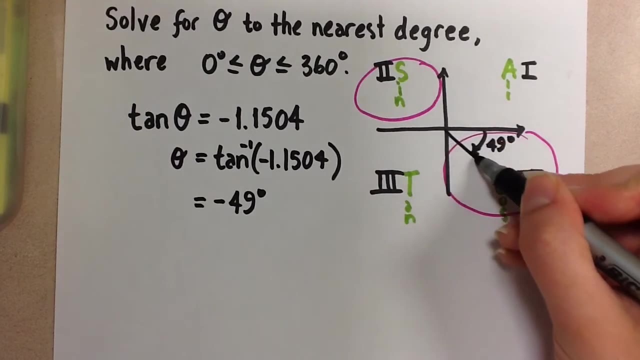 meaning we don't always get principal angles that go counterclockwise. Sometimes we get negative angles And so if we get a negative angle, we're going to go clockwise this way, From the positive X-axis, So the 49 degrees goes here and the terminal arm will land right here in this fourth quadrant. 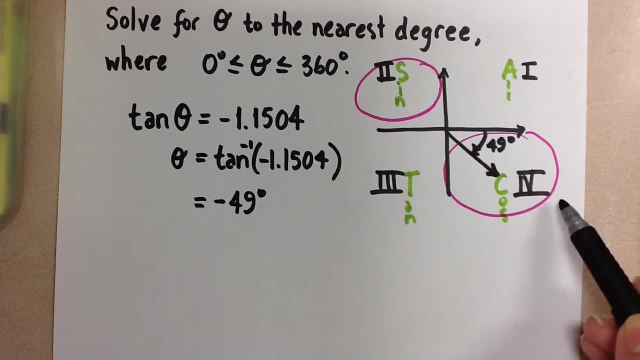 which is correct because we know that the tangent ratio is negative in the fourth quadrant. So there's our first related acute angle there. but we always want to give our answers as positive principal angles. So this negative 49 degrees degrees is not what we want our final answer to be for solving for theta. So we need to. 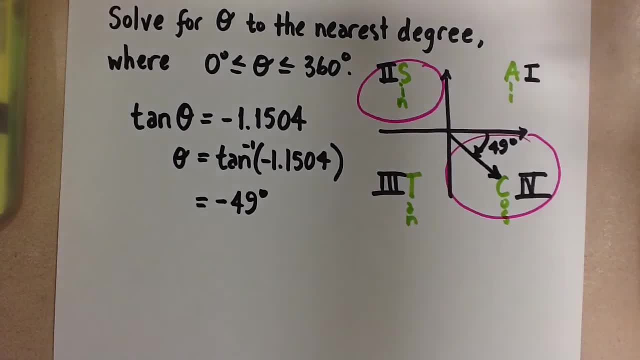 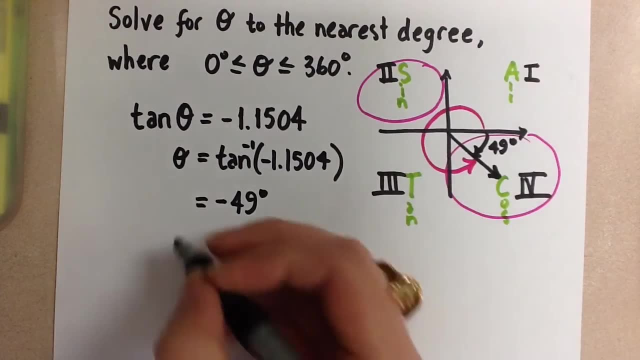 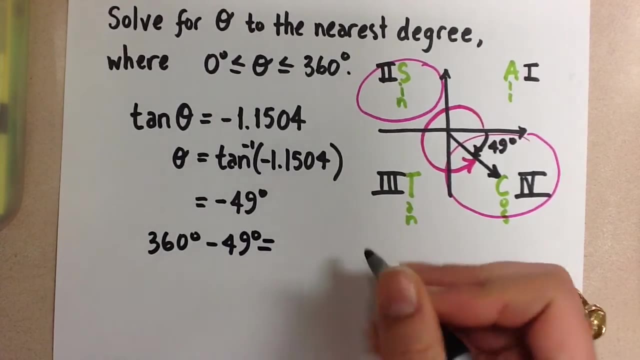 figure out what the principal angle is, or the related angle is that comes around this way like this: So in order to solve for that, we're going to do 360 degrees minus 49 degrees minus 49 degrees and we get 311 degrees. So that's the first solution for this expression. 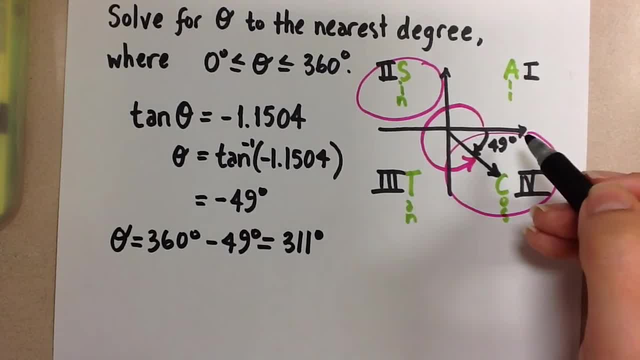 But we know that we need another angle that falls between 0 and 360 degrees and that second angle is going to fall in the second quadrant because that's where the tangent ratio is also negative. So if we have a related acute angle here of 49 degrees, the related 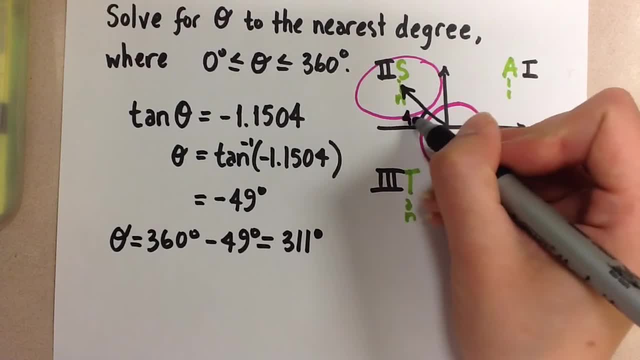 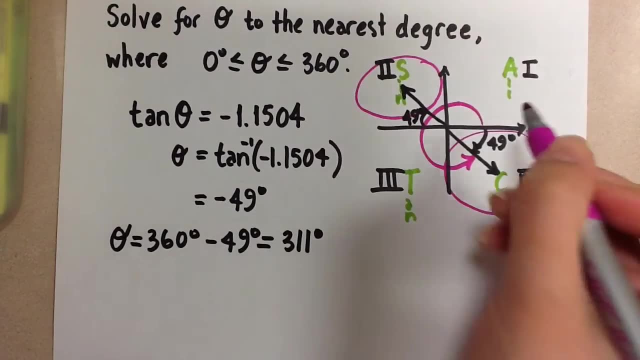 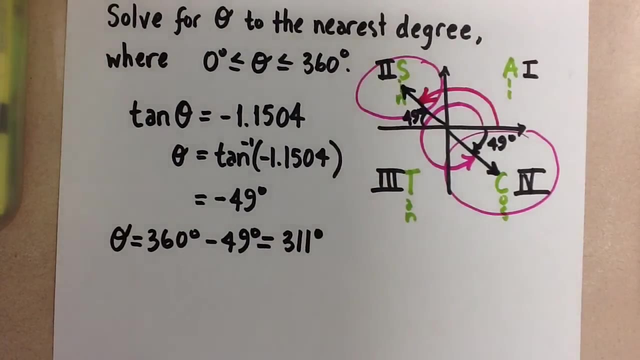 acute angle in this quadrant is also going to be 49 degrees. here And now our job is to find the principal angle made with this terminal arm. So to find that one, we are going to do 180 degrees minus 49 degrees and we get 131 degrees. So that's the first. 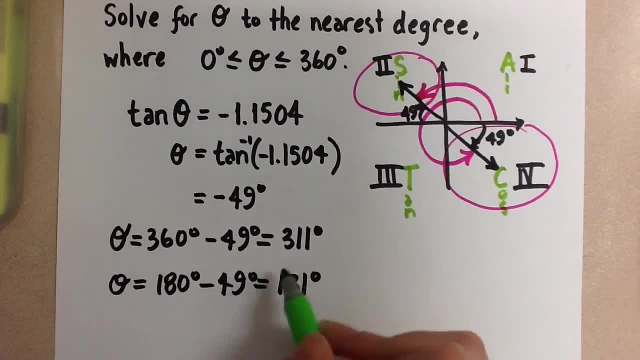 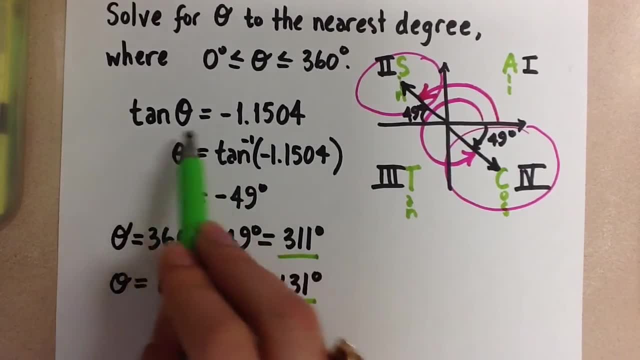 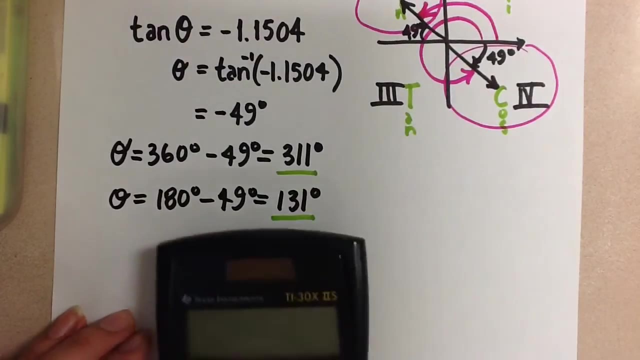 solution for this equation. So our two solutions here are 311 degrees and 131 degrees. So both of these angles should satisfy this equation. We can check this back if you want. You get your calculator and I'll show you how to do that like this, If you get your calculator. 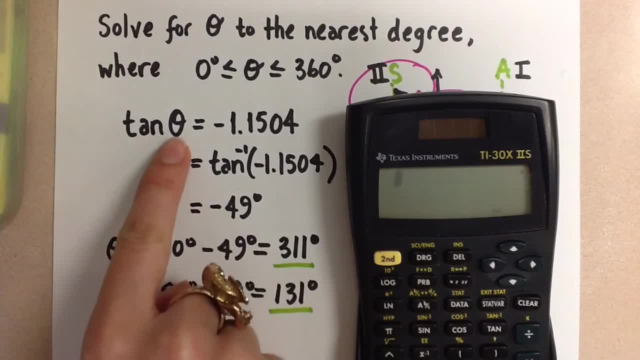 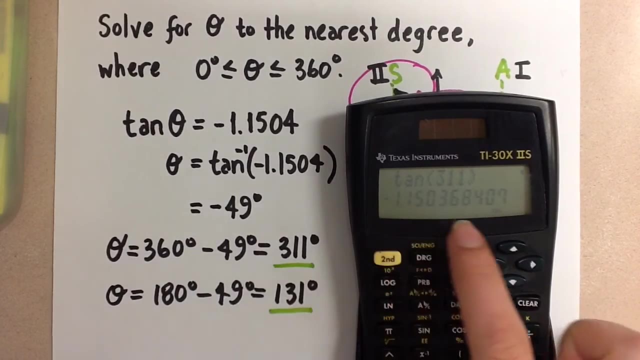 and now we plug in the angle theta that we got here, we should get this negative one, 1.1504 number. So I'm going to do tangent of 311 degrees And there's our answer there, which matches this right side of the equation. So we know that one's correct And we can check. 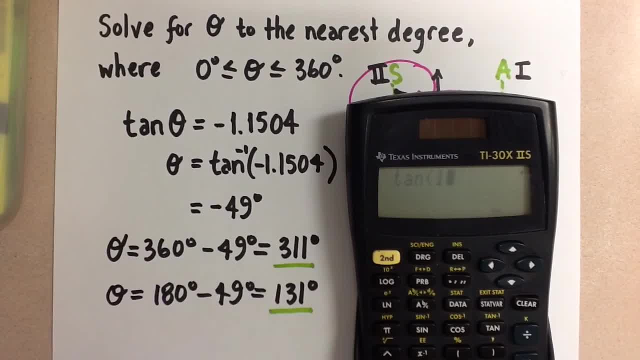 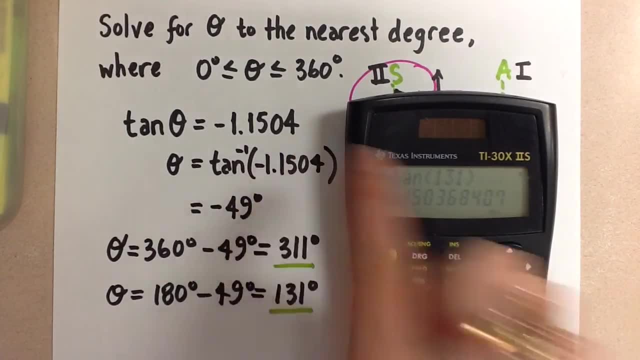 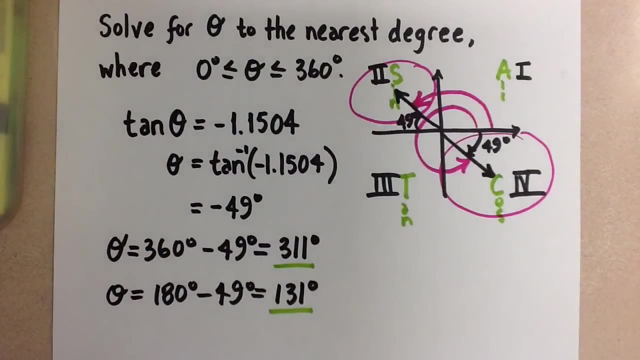 the other one as well. We're going to do tangent of 131 degrees. And there we are again. This is the same as the right side of this equation that we were given initially. So we know that these are the two solutions for this question. Thanks for visiting, Mrs A Loves Math. 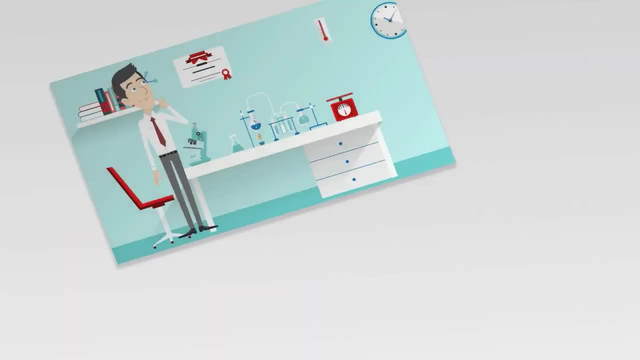 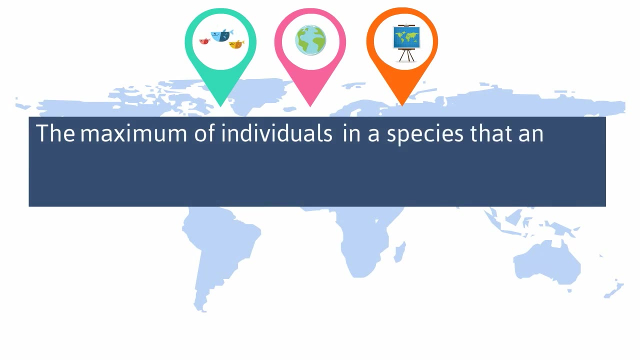 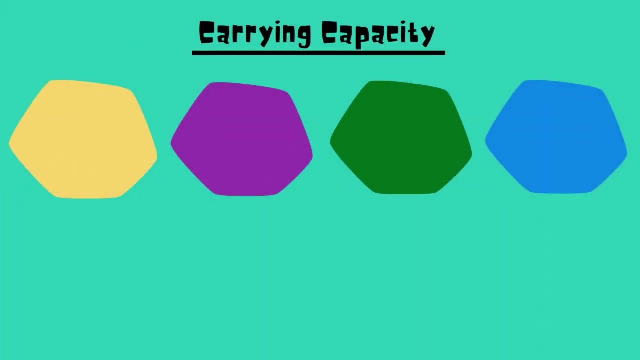 Welcome to MooMooMath and Science. In this video I would like to talk about Caring Capacity of an Environment. The maximum number of individuals in a species that an environment can support for the long term is the caring capacity. Caring capacity is limited by the energy, water, oxygen and space which are all limiting. 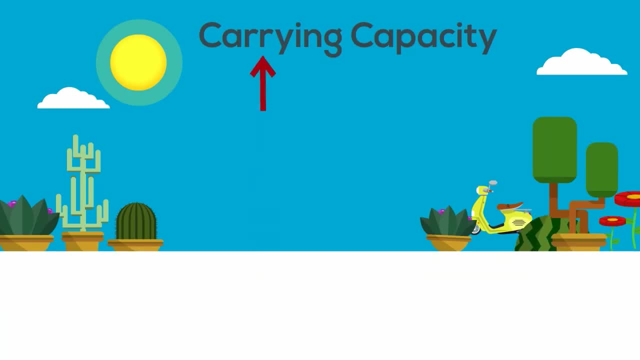 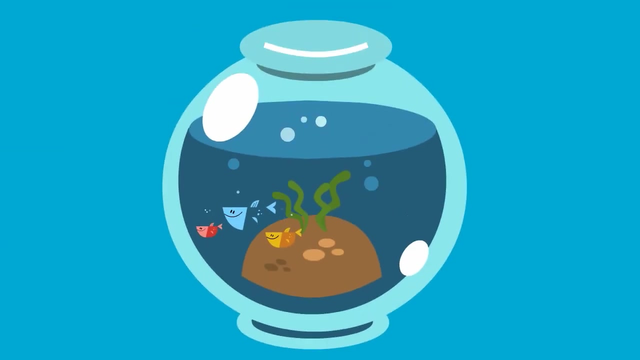 factors. As a population nears the caring capacity, resources become limited. If a population exceeds the caring capacity, deaths begin to outnumber births. Let's take a look at the fish family that live in the fish bowl. Life is plentiful. there's plenty of space, there's food to eat, there's energy from the sun, and they're 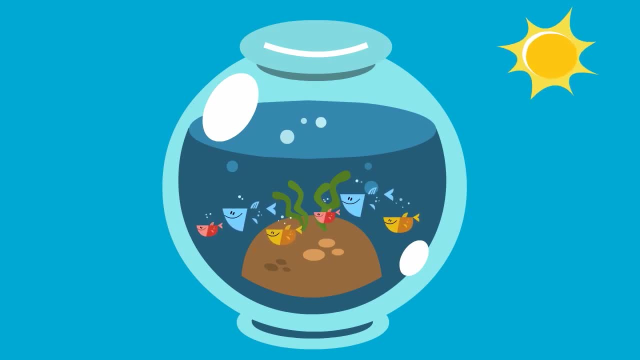 able to reproduce. However, reproduce resources begin to become limited. They are limited by space and the amount of food. However, they are still able to reproduce. Eventually, there become so many fish that some of the fish begin to die off because there is not food to eat. 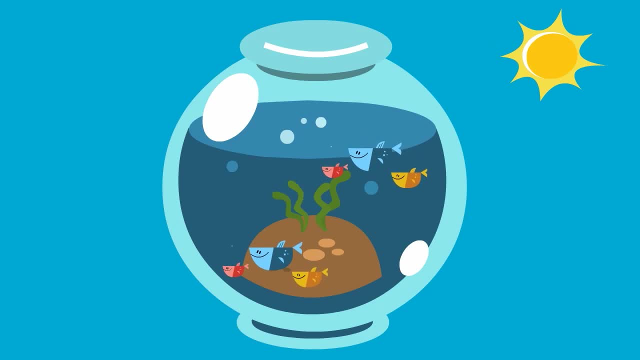 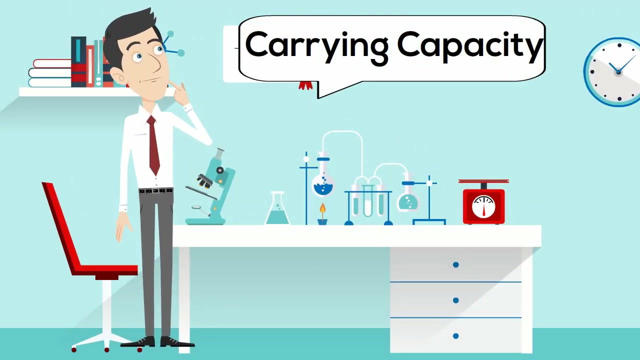 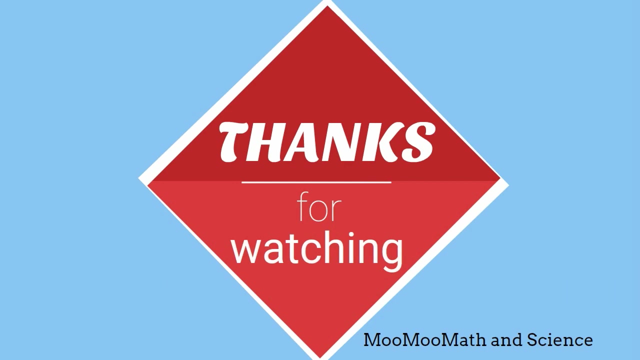 and the water is limited. They have reached the carrying capacity and deaths will outnumber births until it gets back in balance. So there we go. The largest population that an environment can support is known as the carrying capacity. Thanks for watching, and MooMooMath uploads a new math and science video every day.